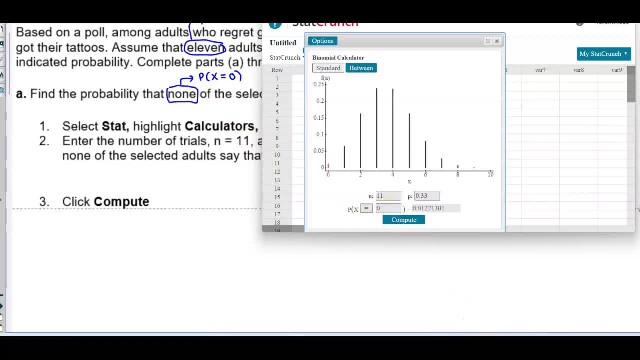 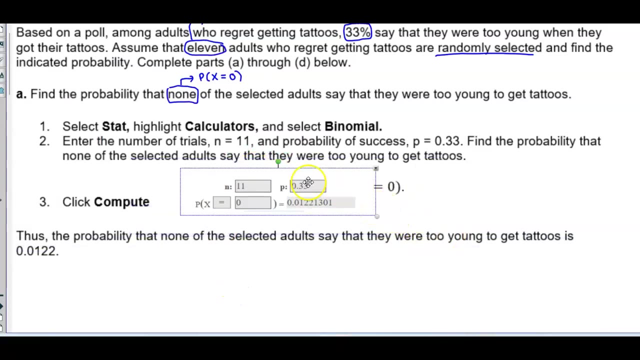 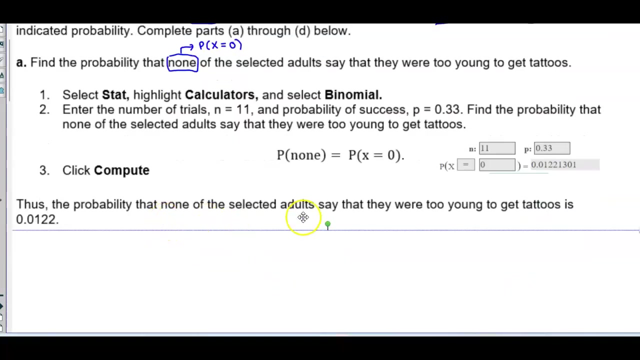 to equal zero, And then select, Compute, And then we have our Okay. so now, rounding this to four decimal places, according to the question, you can see that our probability is 0.0122, thus the probability that none of the selected adults 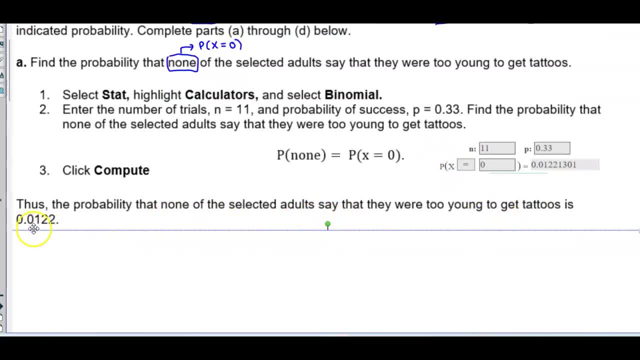 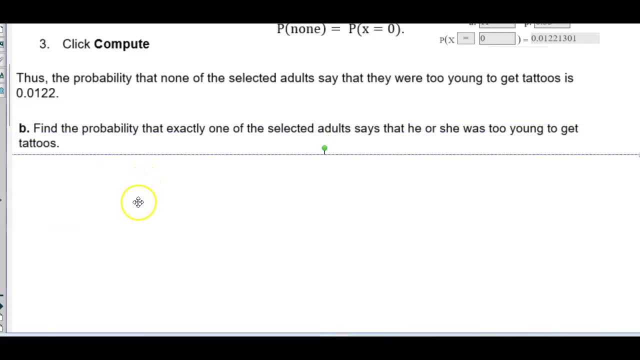 say that they were too young to get tattoos is 0.0122.. Okay, the next question says: find the probability that exactly one of the selected adults says that he or she was too young to get tattoos. Now, exactly one is now telling us that we should now find the probability of when x. 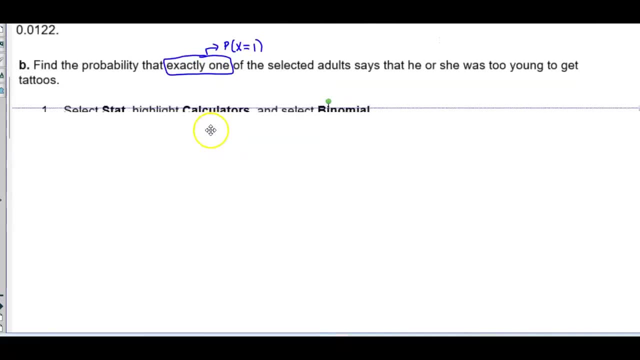 is equal to one. So we're going to be using the same information. We're going to go ahead and select Stat Calculators and Binomial, which we already have. that up in, The number of trials again is 11, p is equal to 0.33, and then we're going to find the 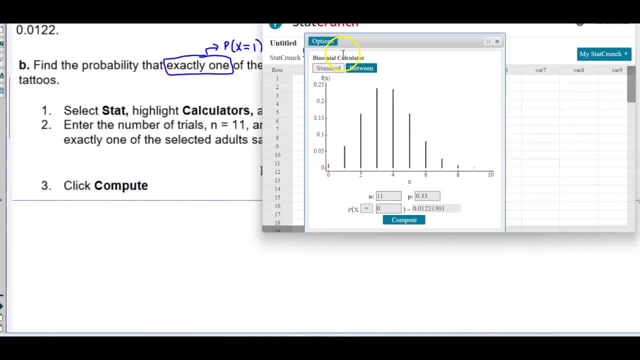 probability of exactly one. So now, all we need to do is find the probability of exactly one. So now, all we need to do is find the probability of exactly one. So now, all we need to do is find the probability of exactly one. So what we need to do is open up Stat Crunch and then change x to be equal to one, because 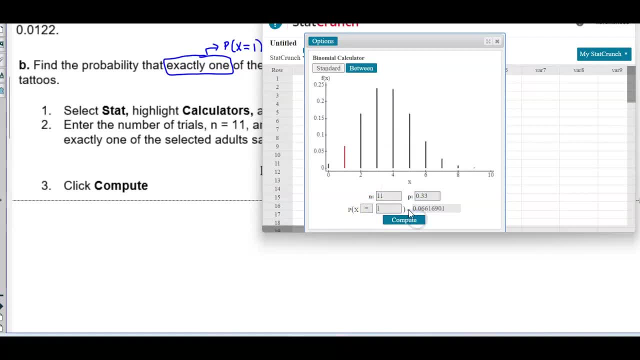 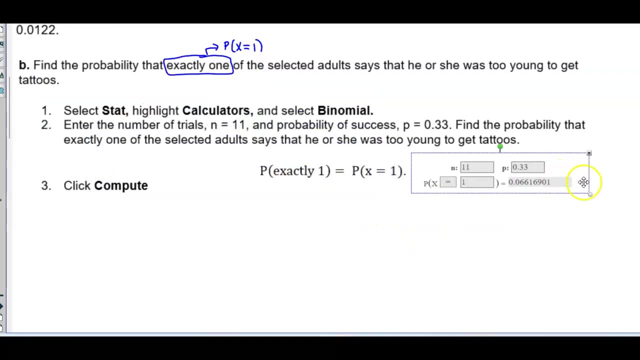 n is already in there and so is p, So let's click Compute and then there we can see the probability of that. So let's go ahead and pull that in. Okay, so we can see what we get there for our probability. So, rounding this to four decimal places, we're going to have to round up that one to a two. 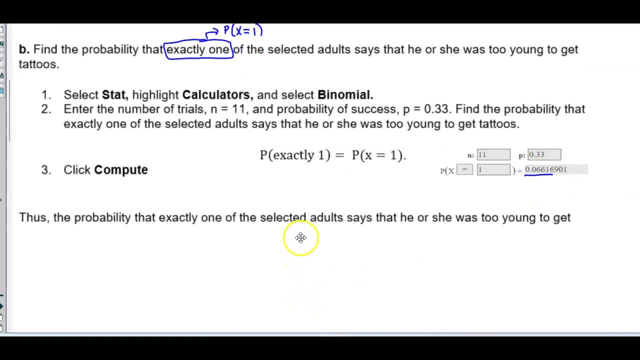 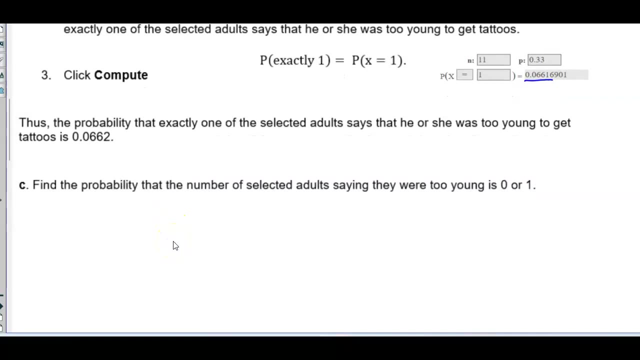 because of the six over here. So therefore, the probability that exactly one of the selected adults says that he or she was too young to get tattoos is 0.0662.. Okay, part C it says: find the probability that the number of selected adults saying they were too young is 0 or 1.. 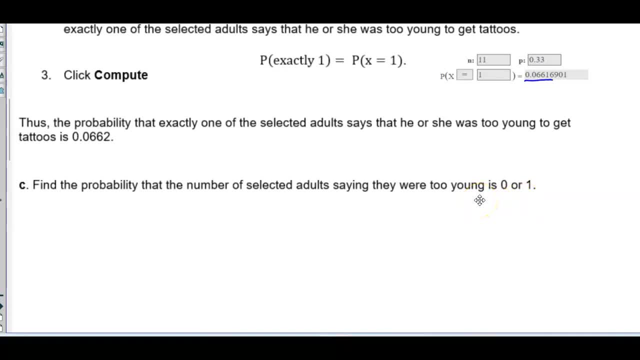 Okay. so one way of doing this is we're looking for the probability that it's 0 or 1.. Another way of saying this is that this is the probability of 0 plus the probability of 1.. Or another way of saying this is that the probability of X being less than or equal to 1.. 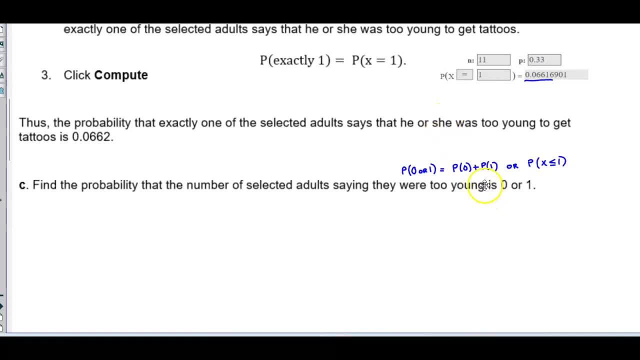 Okay. so there's two ways to go about this: We can use StatCrunch or we can add them together. So let's first use StatCrunch, because, since it says 0 or 1, we're looking for less than or equal to 1.. 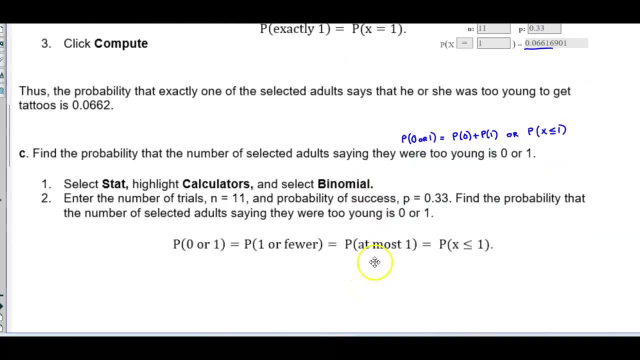 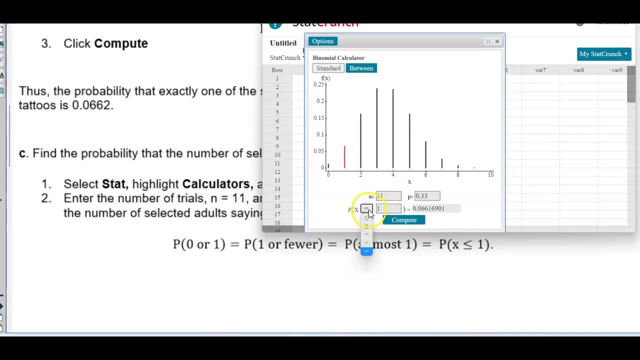 So we're going to go ahead and then put in that information, for when it says 1 or fewer, or X is less than or equal to 1.. Let's go ahead and do that. So in this case here, we're going to go ahead and select less than or equal to 1.. 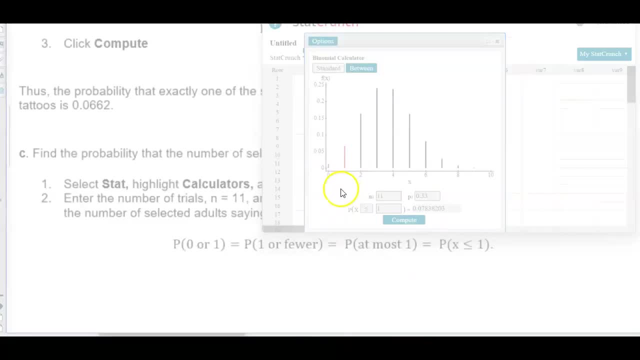 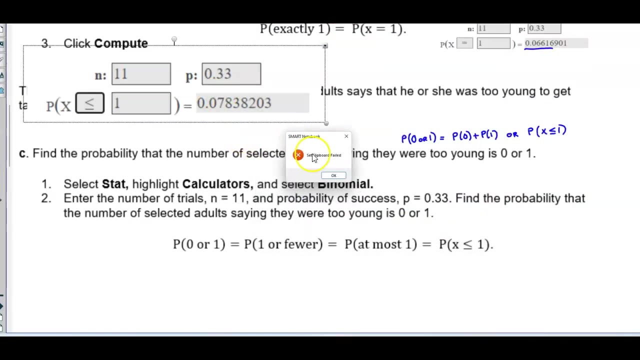 And now we have everything else in there and we can see what the probability is going to be, And it gives us 0.0662.. 0.0783, rounding that to four decimal places is 0.0784.. Okay, now that's going to give us that solution there. 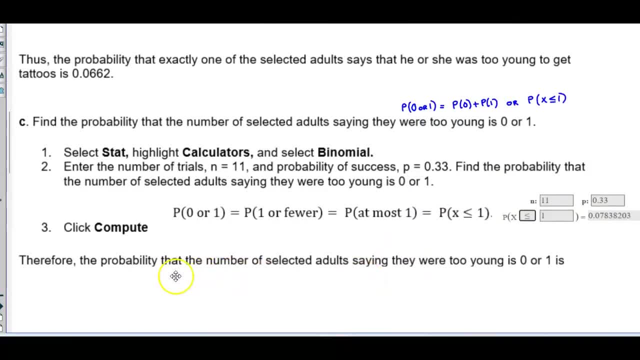 So let's go ahead and take a look here. We say, therefore, the probability that the number of selected adults saying they were too young is 0 or 1 is 0.0784.. Now, what we could have done as well is added those two probabilities. 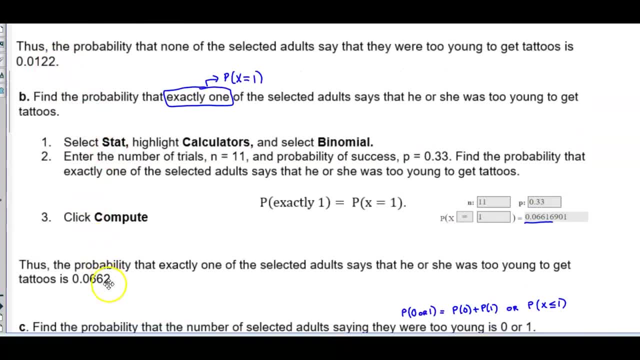 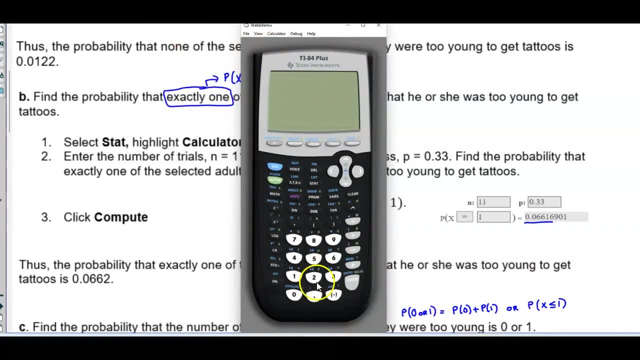 Let's go back. We found the probability of 0 in the first one. We found the probability of the second one. Let's go ahead and see what happens when we add those together, because that's the same thing. So if we take 0.0122 and then add 0.0662,, we get 0.0784,, which gives us the same result. 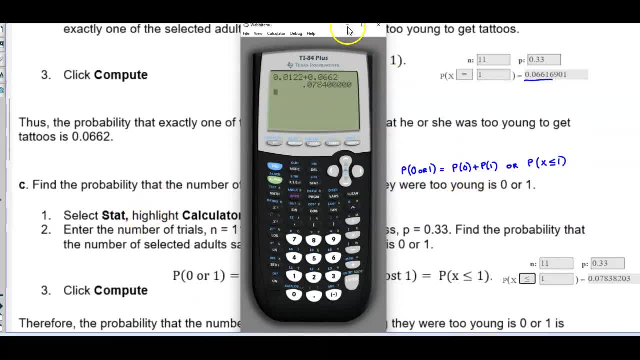 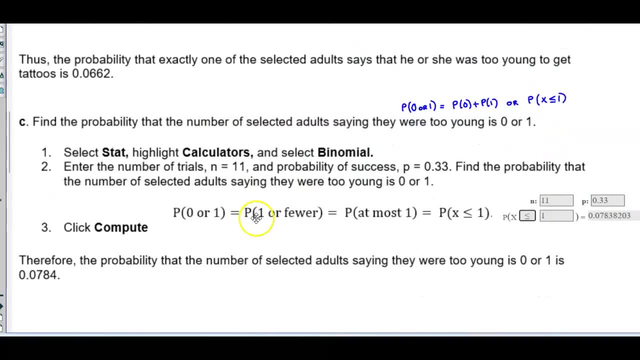 So, either way, you could either add those together. Either way, you could either add those together Using the definition, or you can use StatCrunch and know that the probability of X being less than or equal to 1.. Okay, part D. 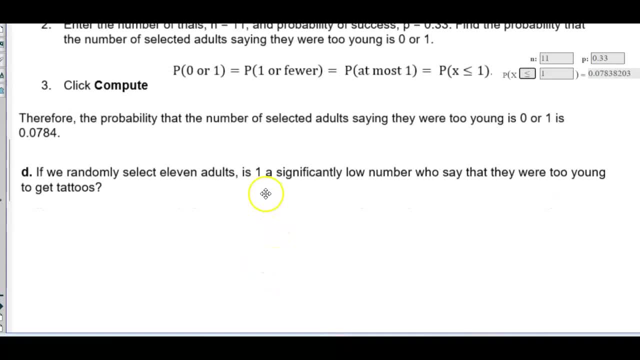 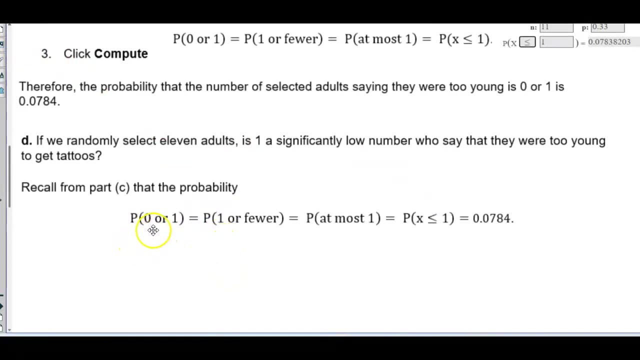 It says: if we randomly select 11 adults, is the probability of 1- a significantly low number- who say that they were too young to get tattoos. Okay, so recall that from part C that we found the probability of 0 or 1,.